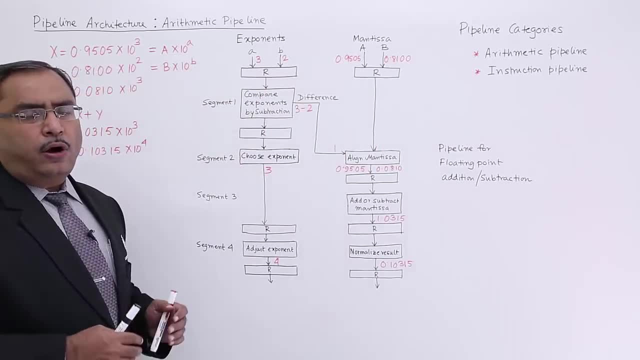 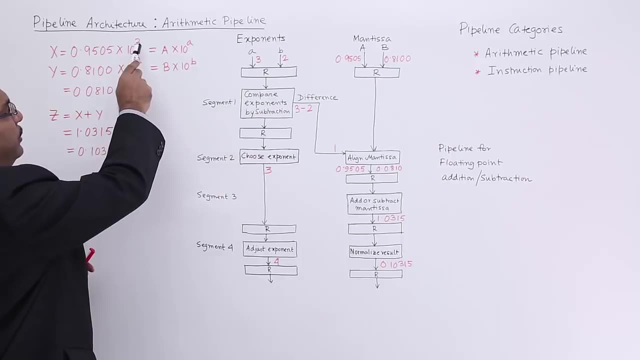 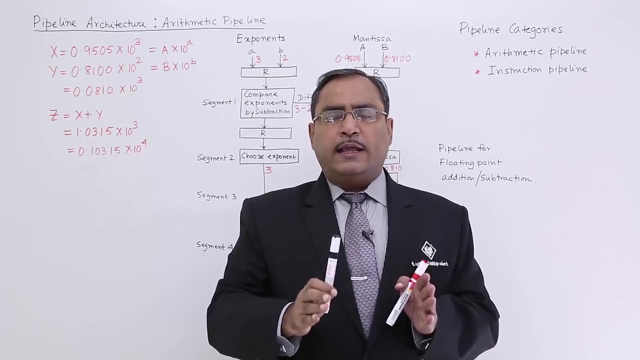 get added. So before adding the significant or mantissa, I should equate the exponent parts. So here we are having this: 3. Here we are having this: 2. Always, it is a common practice to align that very exponent which is having the lesser value to the exponent. 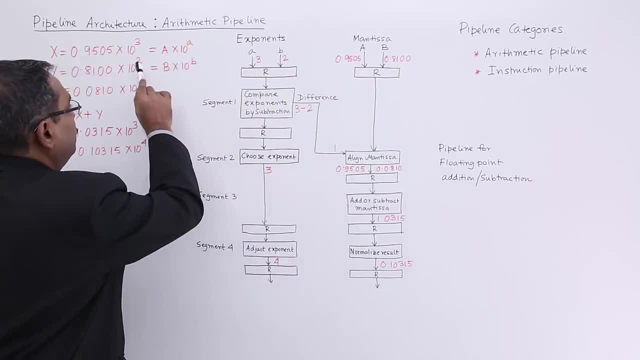 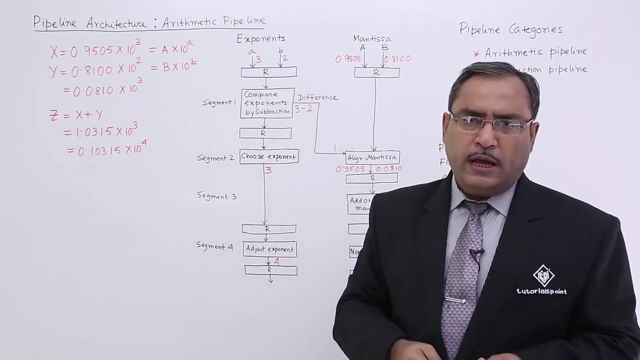 So here the lesser value is 2.. So I want to convert it to the higher value, 3., So that these two exponents will become equal to each other. So for that I had to do some adjustment in the segment in the mantissa significant, And that is quite obvious. So here we have. 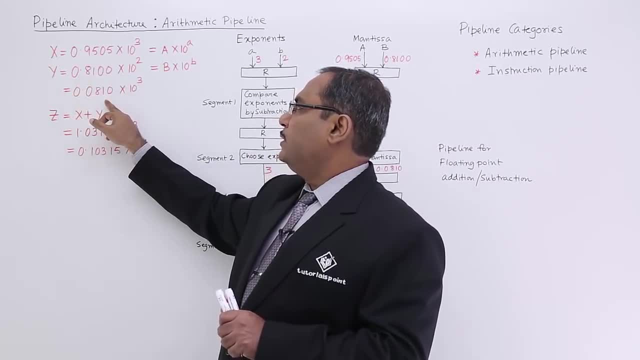 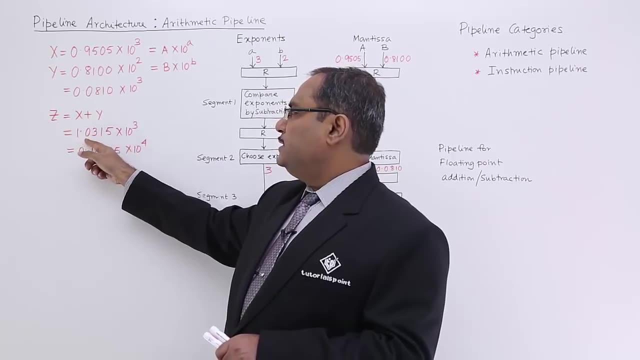 done this, 0.81 has become 0.081.. So now these exponent parts are same. Now obviously we can go for the addition 1.. why i have done so? this is the addition result, that is the sum, and then i have done the normalization. 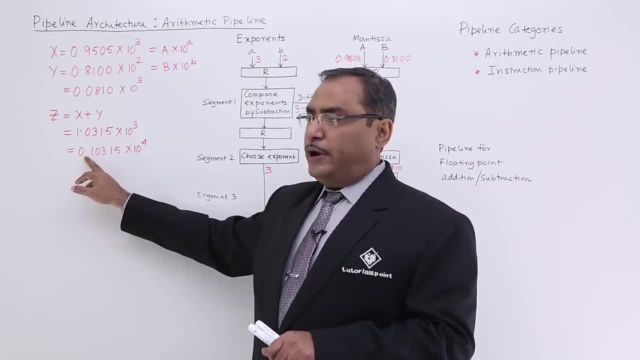 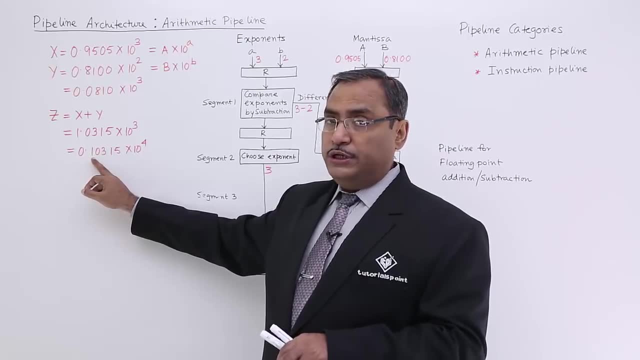 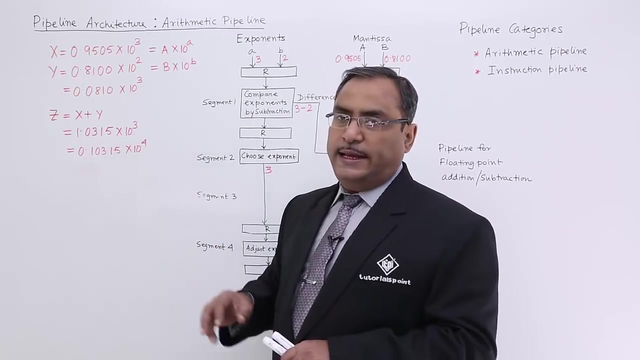 you know, normalization means before this particular radix point, the digit will be 0. after this radix point, the digit will be non 0. two conditions are there for normalization- please see my floating point videos also- and for that purpose you should have to adjust the exponent accordingly. 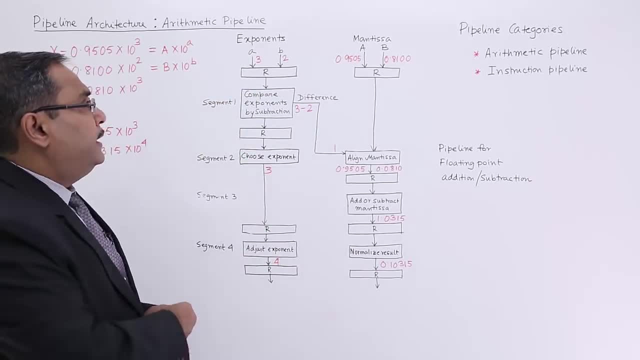 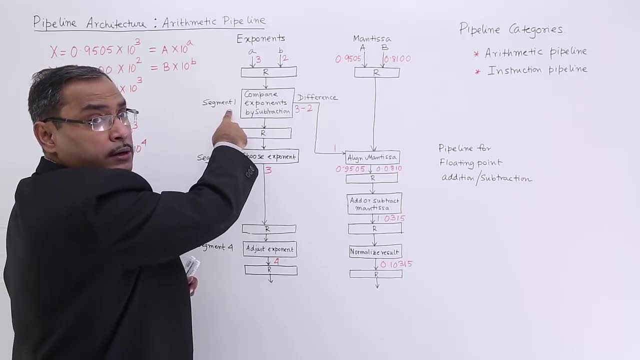 in this particular four segment pipeline i have depicted the same. here they are taking this exponent, here they are taking the mantesa. now comparing exponent will be of segment number 1. so what i am doing, i am doing just a minus b. what i am doing, i am just doing. 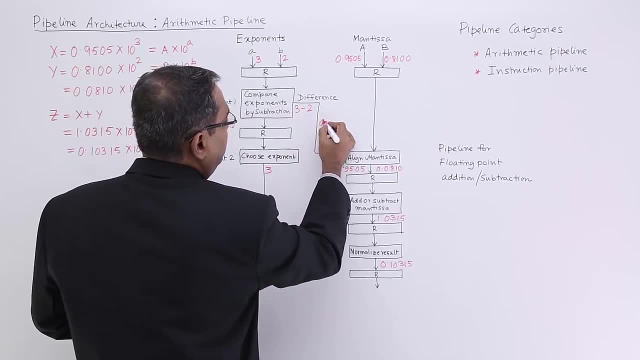 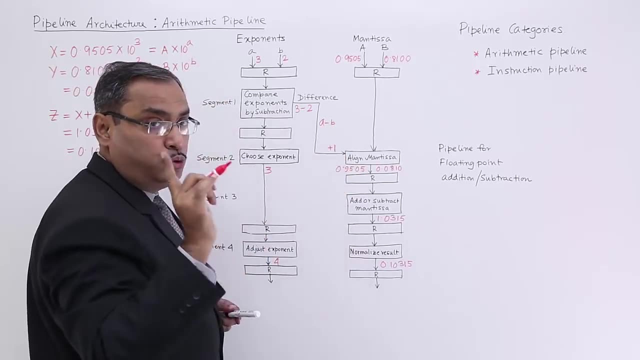 just a minus b. so when i am doing a minus b, then what will happen? here? i am getting 1, so 1 is a factor and another factor is plus 1. two things are there. 1 is, 1 is the value for A, 2 is the jail point. 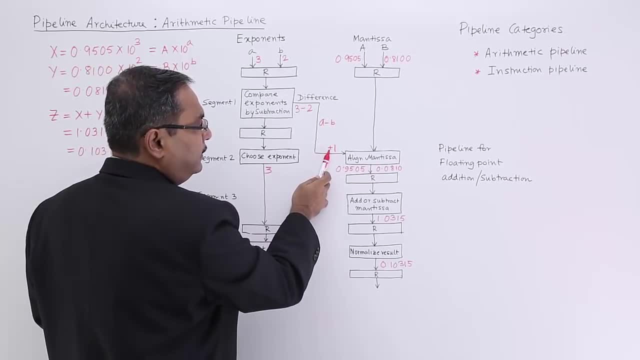 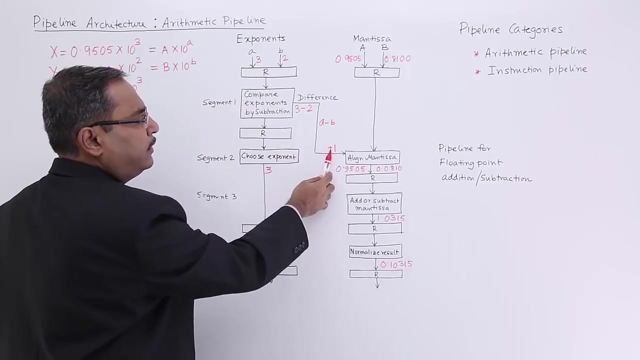 another one is a sign. The sign will indicate that I should adjust the second exponent part, and this magnitude will indicate that I should adjust it for 1 plus. So that is why if it is minus 1, then obviously I should consider this first exponent, that is a in that case. So in this,